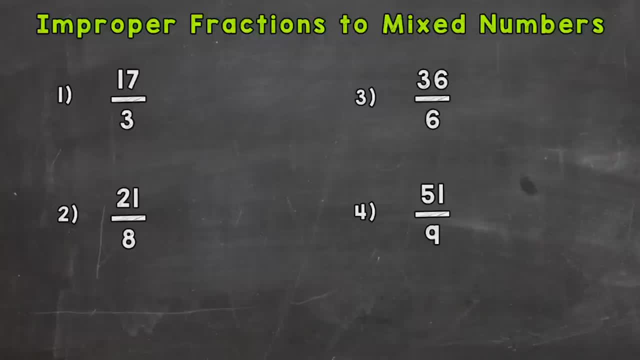 you're ready and check your answers with mine. Let's hop right in to number one. In number one we have 17 thirds, or 17 over 3.. So we're going to take all four of those and convert them to mixed numbers. 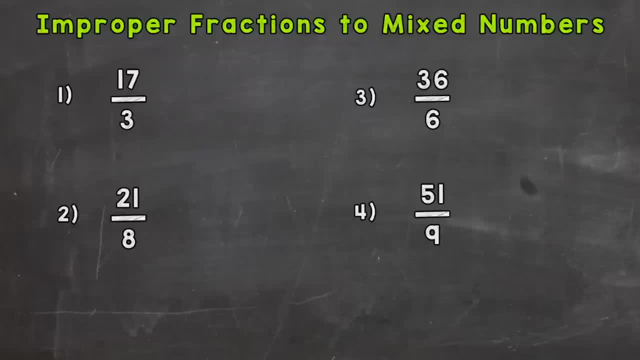 So, as you can see, there are four problems on your screen, four improper fractions. we're going to take all four of those and convert them to mixed numbers. need to convert that to a mixed number. in order to do so, we need to divide. we. 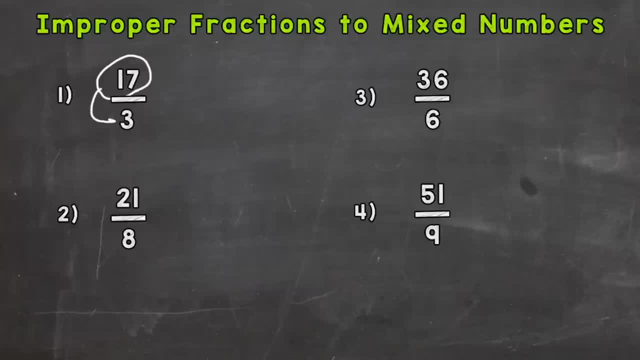 take the numerator, the 17, and we divide it by the denominator. so I'm going to set up a problem over here to show exactly what I'm doing. so we need to do 17 divided by 3. how many whole groups of 3 can we pull out a 17? hopefully you're. 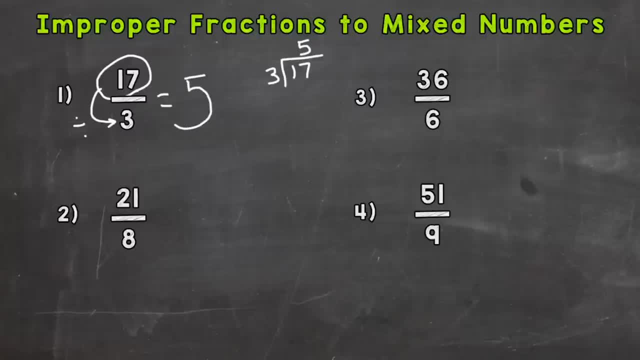 thinking 5 whole groups, so that's our whole number for the mixed number, for our answer. so it doesn't work out exactly. there's going to be a remainder. so 5 times 3 is 15 subtract and we get 2 left over. so whenever there is a remainder it's the 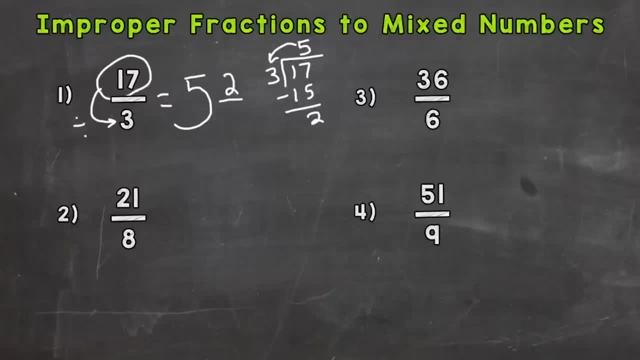 numerator portion of the fractional part of the mixed number. so we put our 2, our remainder, up here and then we keep the denominator the same, you don't need to change it. so we get 5 and 2 thirds. so again the division problem, 17 divided by: 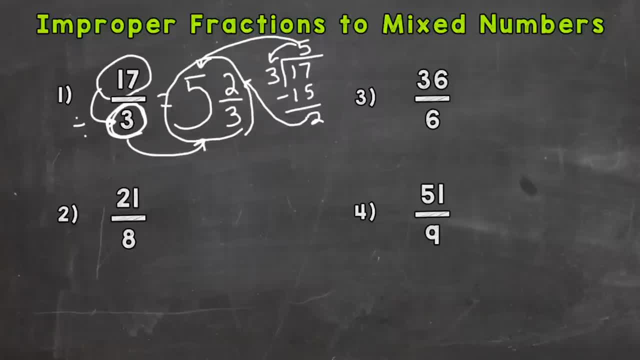 3, the whole number, we got 5 the remainder. we got this 2 right here and we keep the denominator the same. so let's hop over to number 2 or down to number 2: 20 divided by 2, 21, eighths. so the first thing we need to do is divide 21 by 8 and once you get, 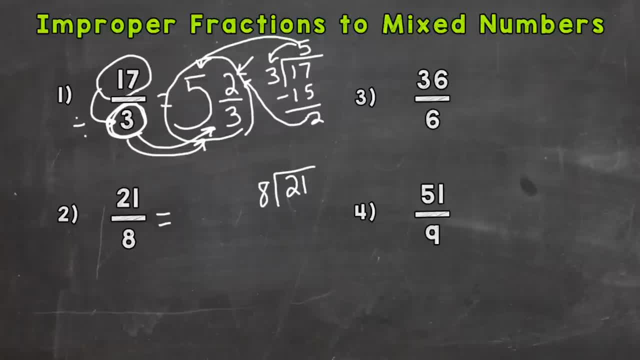 good enough at these and you're very comfortable with them. you won't need to write out the division problem. some of you may be to that point already. so, 21 divided by 8, how many whole groups of 8 can we pull out of 21? well, 8, 16, 24, 3, 8, 3. 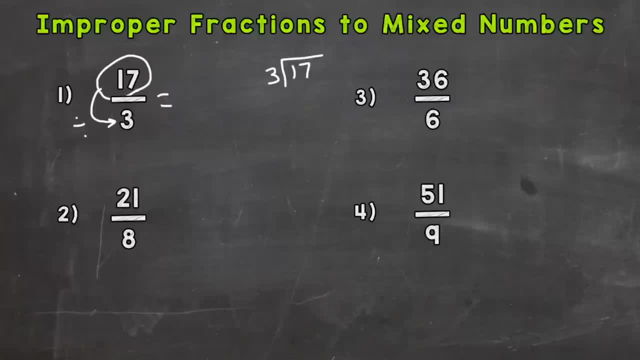 How many whole groups of 3 can we pull out of 17?? Hopefully you're thinking 5.. We're going to do 5 whole groups, So that's our whole number for the mixed number for our answer. So it doesn't work out exactly. 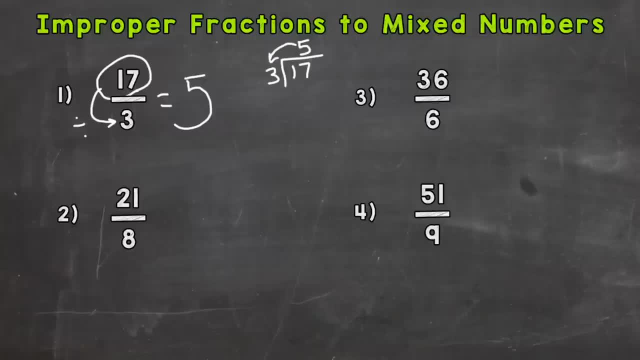 There's going to be a remainder. So 5 times 3 is 15.. Subtract and we get 2 left over. So whenever there is a remainder it's the numerator portion of the fractional part of the mixed number. So we put our 2.. 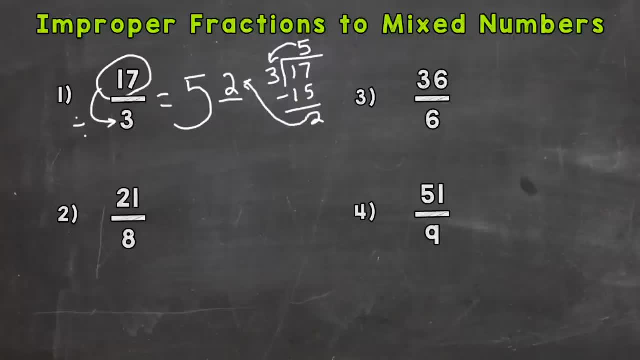 Our remainder up here. And then we keep the denominator the same, You don't need to change it. So we get 5 and 2 thirds. So again the division problem: 17 divided by 3. The whole number, we got 5.. 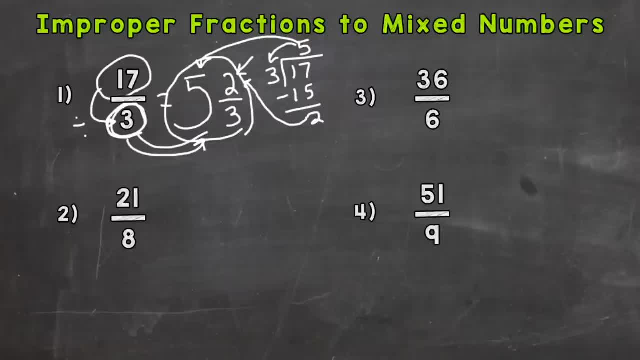 The remainder. we got this 2 right here And we keep the denominator the same, So let's hop over to number 2 or down to number 2.. The whole number we got is 21 eighths, So the first thing we need to do is divide 21 by 8.. 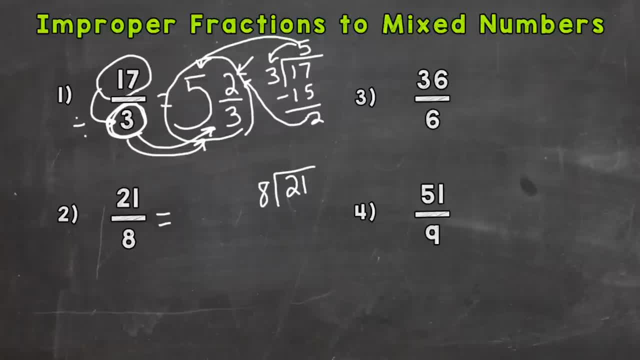 And once you get good enough at these and you're very comfortable with them, You won't need to write out the division problem. Some of you may be to that point already. So 21 divided by 8.. How many whole groups of 8 can we pull out of 21?? 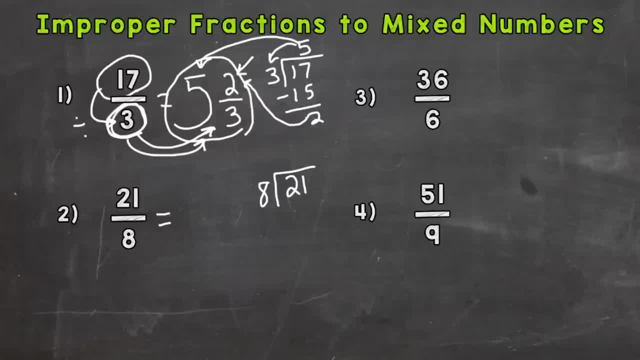 Well, 8, 16, 24.. 3 eighths 3 eighths 20.. So it's only going to be 2.. So that's our whole number. part of our mixed number, 2 times 8, is 16.. 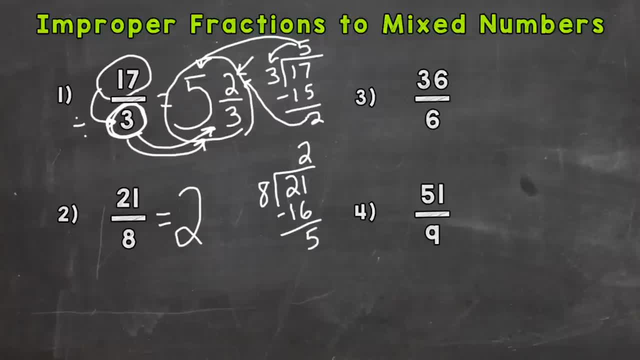 We subtract and we get a remainder 5.. So, remember, the remainder is our numerator portion of the fraction. And then we keep the denominator the same. So 2 and 5, eighths Number 3, we have 36 sixths. 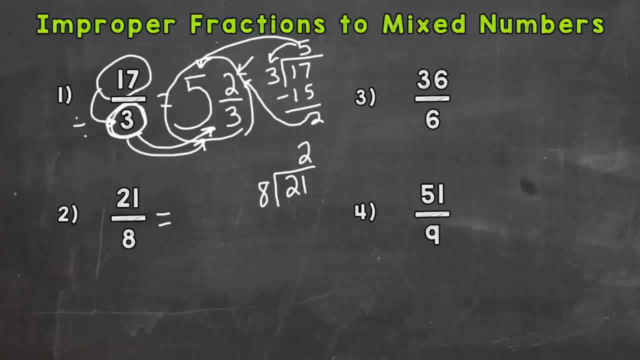 8 is too many. so we're going to have to divide 21 by 8. so we're going to have to divide that as well. so we're going to go back into the integral and we multiply it over and multiply each as many as possible twice and we'll get quiadia. 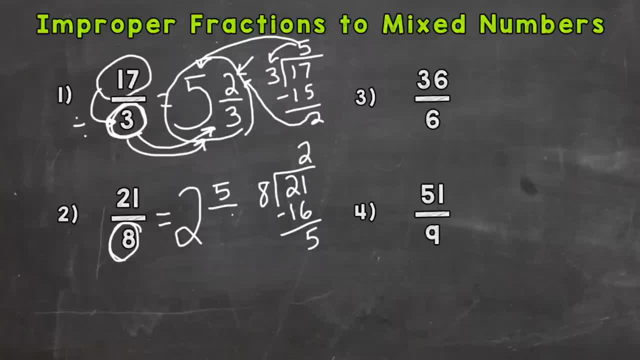 內 is finished in the next part. so now we get moto n, but we just left the numerator, so we get 2 times 8 and we get 2 sixteen. lets try this one real quick, because I'm an old man, I'm not going to put alphabets all the times and times 6, as in taixel. 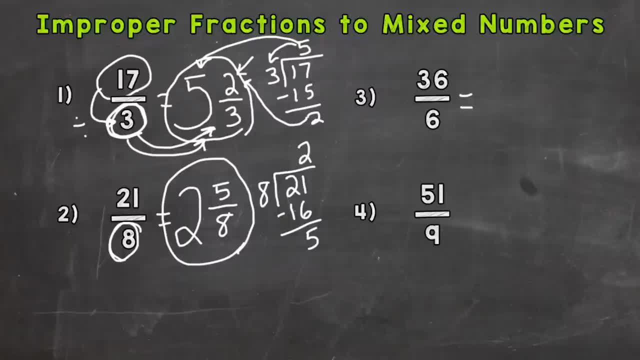 Number three: we have 36 sixths, so 36 over 6.. So the first step is divide. We need to do 36 divided by 6. And so we need to think how many whole groups of 6 can we pull out of 36?? 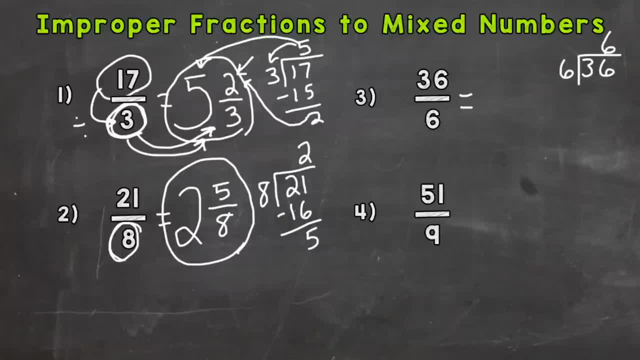 And the answer to that is 6, right, And we hit 36, exactly 6 times 6, 36.. And we do not get a remainder. So our answer is going to be 6 wholes. If there's no remainder, you're just going to have a whole number. answer so: 6.. 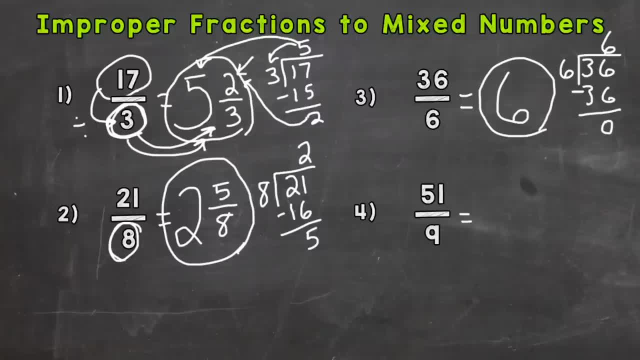 Number four: 51, ninths, 51 over 9.. So we need to do 51, we'll come down here divided by 9. How many whole groups of 9 in 51?? Well, 5.. That gets us to 45.. 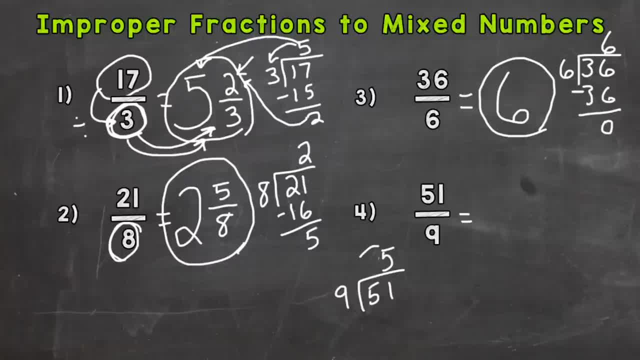 If we do 6 groups, that's too many. So 5 times 9 is 45. Let's subtract to see what the remainder is going to be. 51 minus 45 is 6. So we get 5 wholes. 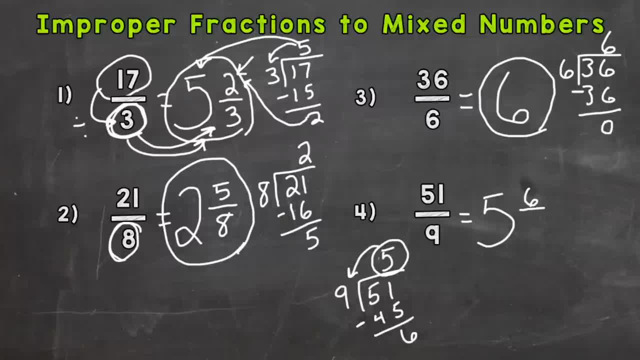 We have a remainder of 6. And we keep the denominator the same. So 5 and 6 ninths. Now let's do the denominator. Let's do the denominator. Let's do the denominator, Now that 6- ninths can actually be simplified, because we have a common factor between 6 and 9 other than 1.. 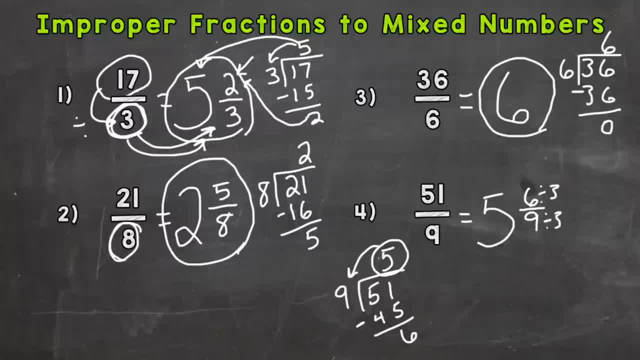 So we can divide both the 6 and 9 by 3. to break it down: 6 divided by 3 is 2. And 9 divided by 3 is 3.. So we can actually rewrite our answer as 5 and 2 thirds. 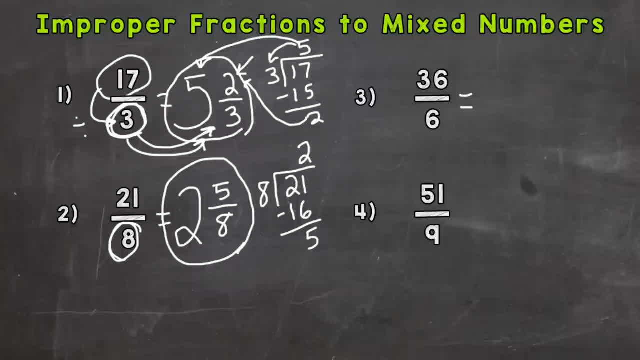 So 36 over 6.. So the first step is divide. We need to do 36 divided by 6.. And so we need to think how many whole groups of 6 can we pull out of 36? And the answer to that is 6.. 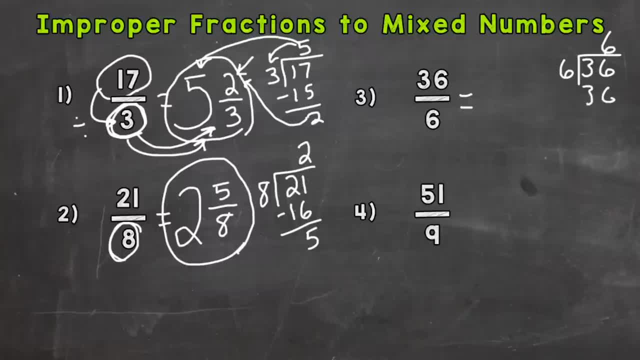 And we hit 36 exactly 6 times 6 is 36. And we do not get a remainder. So our answer Is going to be 6 wholes. If there's no remainder, You're just going to have a whole number answer. 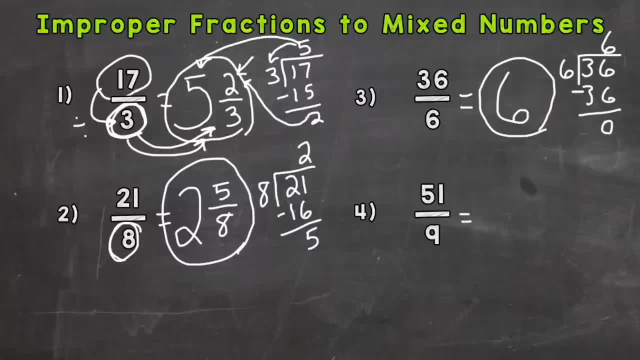 So 6. Number 4.. 51, ninths 51 over 9.. So we need to do 51.. We'll come down here Divided by 9. How many whole groups of 9 in 51?? Well, 5.. 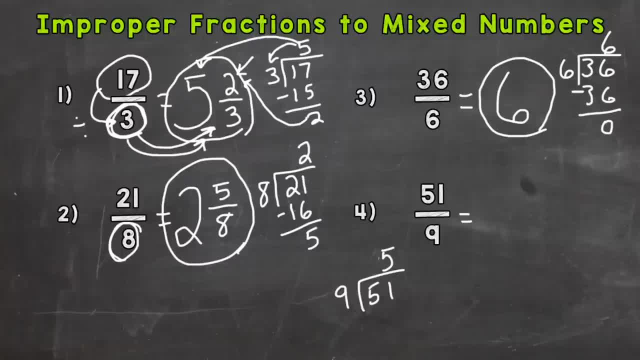 That gets us to 45. If we do 6 groups, That's too many. So 5 times 9 is 45. Let's subtract to see what the remainder is going to be. 51 minus 45 is 6.. 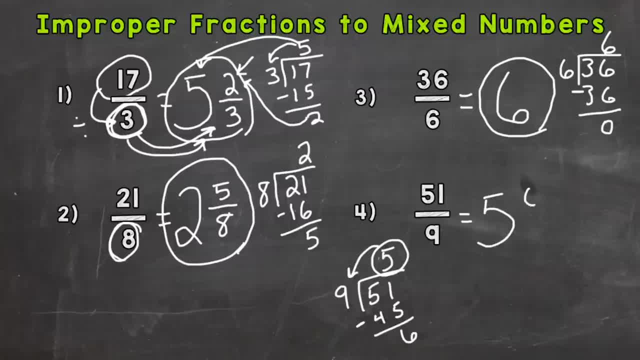 So we get 5 wholes, We have a remainder of 6. And we keep the denominator the same. So 5 and 6 ninths. Now that 6 ninths Can actually be simplified Because we have a common factor between 6 and 9.. 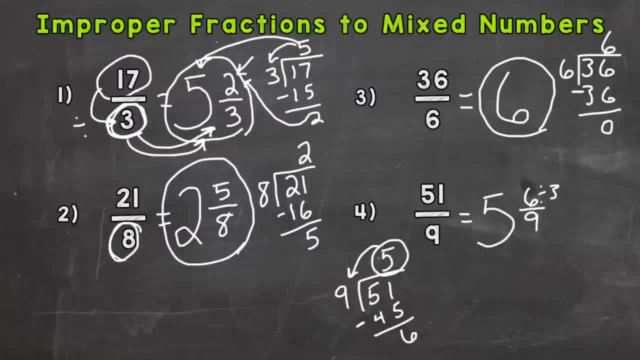 Other than 1.. So we can divide both the 6 and 9.. By 3. to break it down: 6 divided by 3 is 2. And 9 divided by 3 is 3.. So we can actually rewrite our answer as 5.. 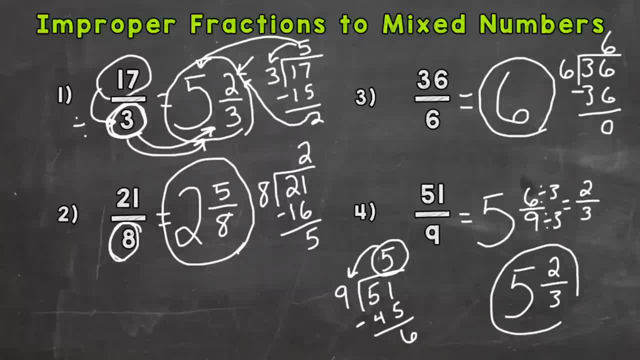 And 2 thirds. We simplified the fractional part Of the mixed number Alright. So that's how you convert improper fractions to mixed numbers. All it is is division And then rewriting your whole number, remainder and denominator in the correct places. 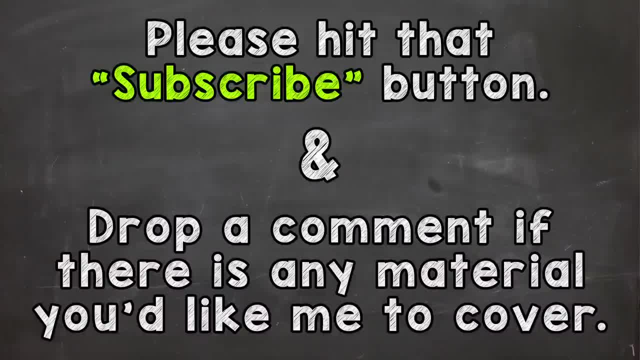 Thanks so much for watching. Until next time, Peace.